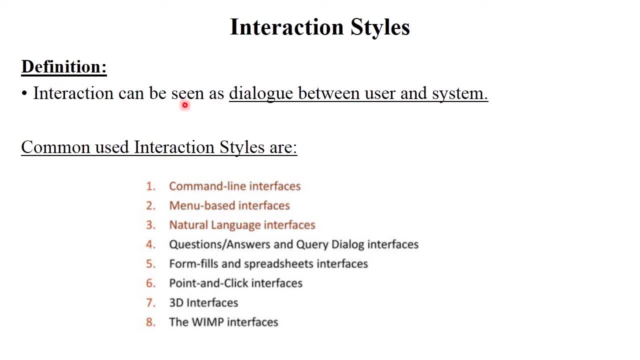 Styles. The definition of Interaction Style. Interaction can be seen as dialogue between user and system. simply Interaction means communication, dialogue between user and the system or human and the system, which is called as Interaction. There are total 8 common used Interaction Styles which included also in your syllabus: Command Line Interface Menu. 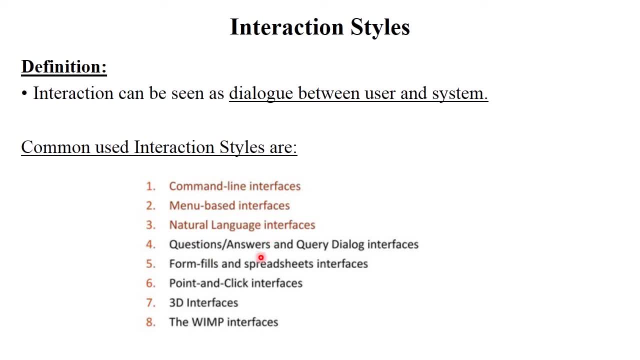 Based Interface, Natural Language Interface. Question Answers and Query Dialogue Interface. Question Answers and Query Dialogue Interface. Form Fills and Spreadsheet Interface, Point and Click Interface, 3D Interface and WIMP Interface. These are all the Interaction Styles. So in this video we will learn about first 4 Interaction, That is, Command Line Menu. 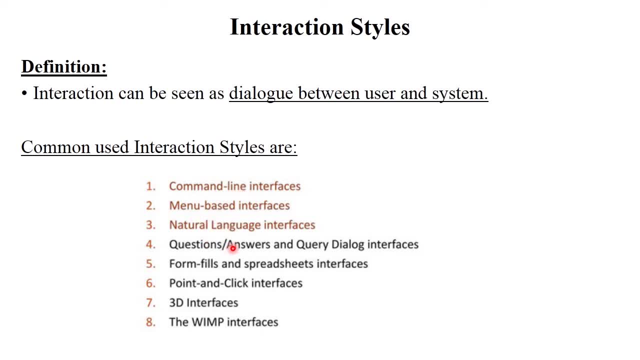 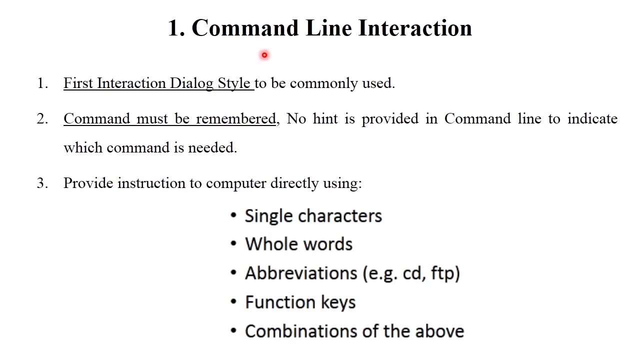 Based Natural Language and Question and Answers. Next, 4 Interaction Styles we will learn in my next video. that is part 2.. Clear, So let's see one by one. Next, So first Interaction Style is Command Line Interaction. It is a first Interaction Dialogue. 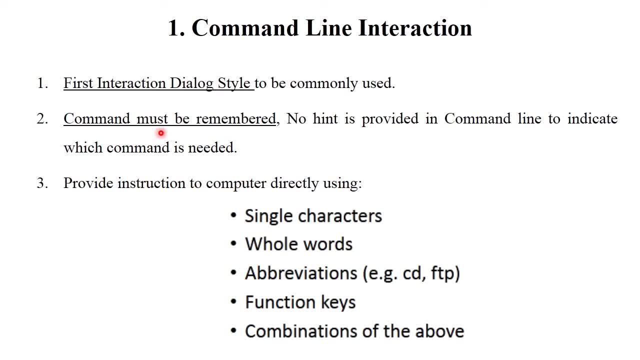 Style which commonly used. By using Command Line Interaction, you have to remember each and every command. No hint is provided in Command Line to indicate which command is needed. It provide a instruction to computers directly using single characters, whole word, abbreviations, function keys, combination of the above. Let's see one example of Command. 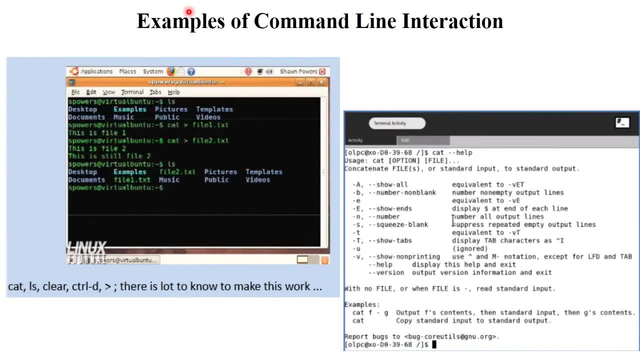 Line Interaction Next. Ok, You all are familiar with the Command Prompt, which is also called as Command Line Interaction, By using Command. Now see here: In this Command Prompt ls command is used. ls command is used for show all the folders in your computer. Then cat command for file purpose. Ok, Also. 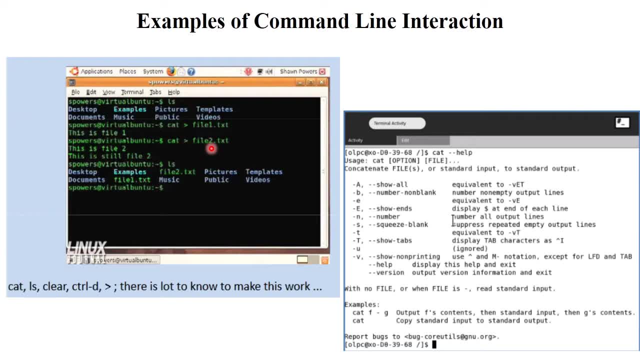 there is a command for showing all the folders in your computer, Then cat command for file purpose. Ok, Ok, mkdrm, make directory command is used in this way. there are particular command is used clear by using command prompt. you have to access each and every files by using command clear. 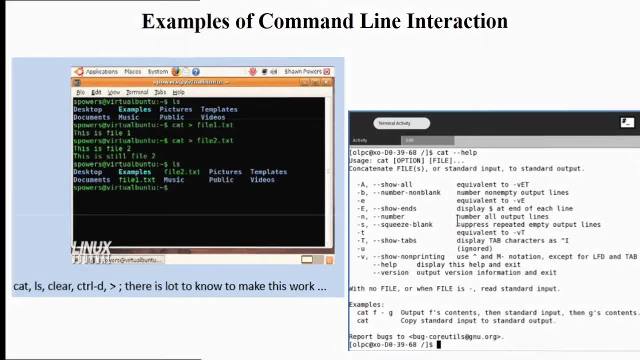 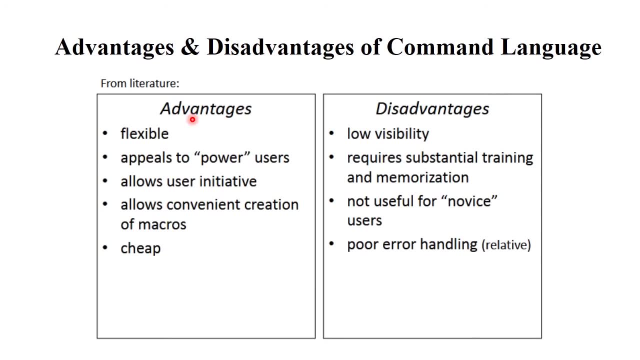 this is the example of command prompt. next, there are also advantages and disadvantages of command languages. the advantages of command line interface which is flexible, which appeals to power users, means the technical users only used this command prompt. normal users or the people who is not in technical background. 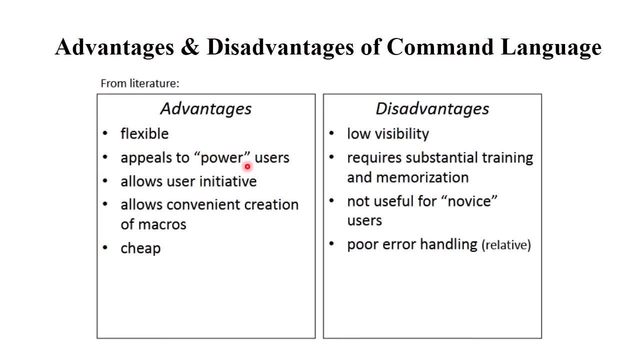 they don't use this command prompt because it required the proper knowledge of each and every command. it allow users initiative, allow convenient creation of micros and also chip. micro means functions. it also create different programming in linux learning system. it also create different operating system. they use all those linux commands. ok, now the disadvantages. 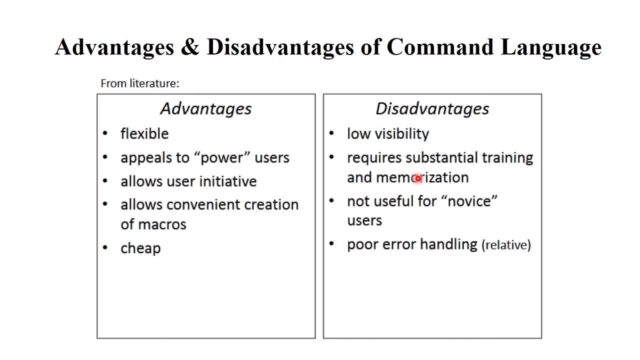 of command line interface which has low visibility. it required substantial training and memorization. you have to memorize or remember each and every command regarding the particular situation. which is not useful for novice users means it is useful only for technical person. poor error handling: ok, there is also error handling ok. 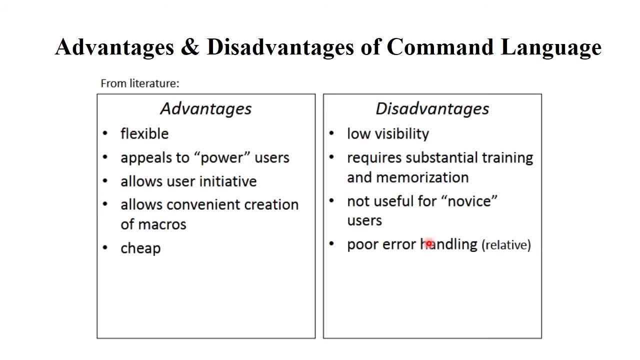 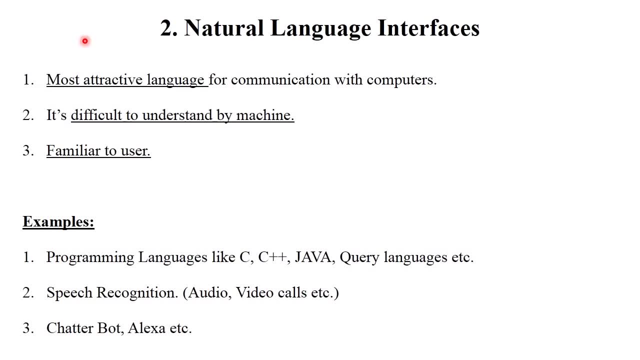 there is also error handling. ok, there is also error handling, ok. exam: nt6 exam. nt7 exam. nt8 exam. nt2 exam. nt7 exam. 12 exam, nt11 exam n. still its 5th mercy, Jen. the these might be be consider more powerful that are practical, but check the finished. 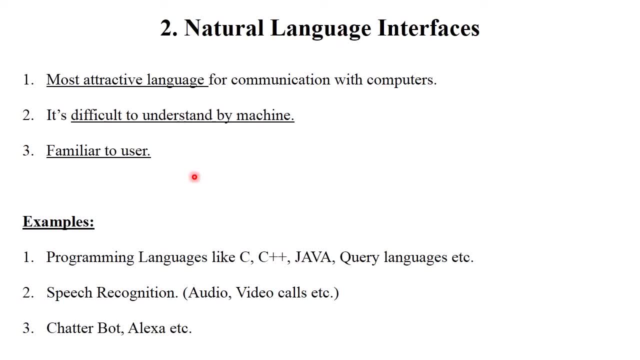 below: okay, ok, so by the user, not the machine. each and every machine understand the binary language. binary language is always in 0, 1: 0 format, clear, so natural language interface is familiar to the user. for example, programming languages like C, C plus plus, Java, any query languages, etc. in all the programming language we used. 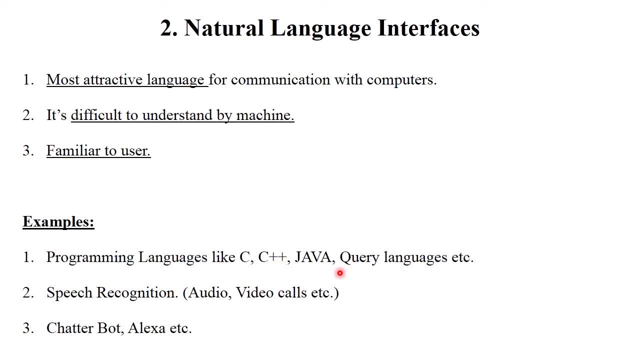 a natural language, for example English. we used English language in this programming or while implementation. clear against speech recognition. for speech recognition, we used audio and video calls. okay, for that purpose we also use natural language. then chatbot, Alexa, different types of robotics app, also design clear. this is called as natural language interface. next, now see. 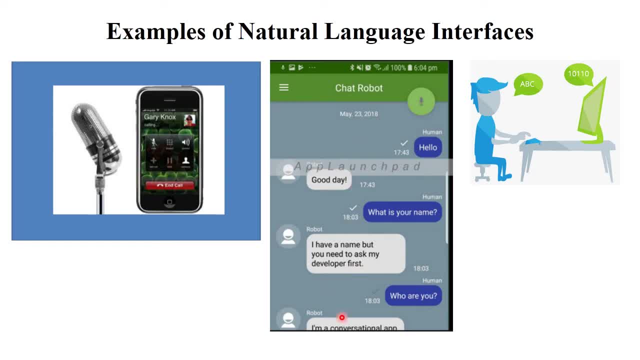 the examples of natural language interface: the chat robot: okay, we have to chat in our own language here. then audio call and voice call: we use our own language. now, as see this, we have to type a, B, C using keyboard and this ABC pass to the system, but this: 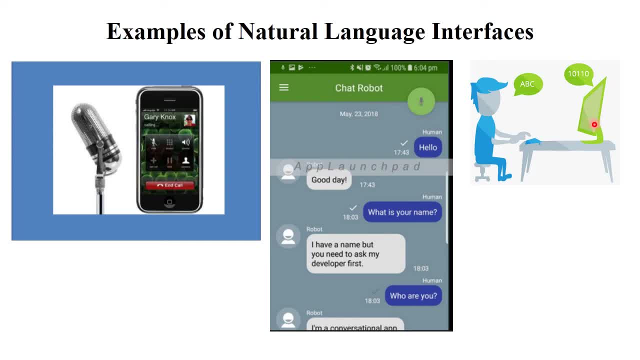 English language or natural language does not understand by the computer. so computer tech is in binary format like one zero, one, one zero. so keyboard system are already built in or implemented in that way. clear. so ABC is a source language or natural language and one zero, one, one zero. it is the machine. 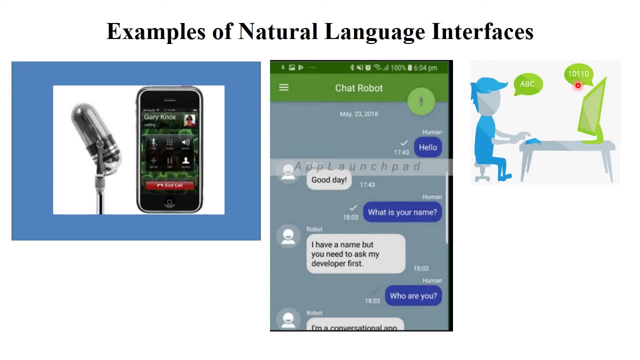 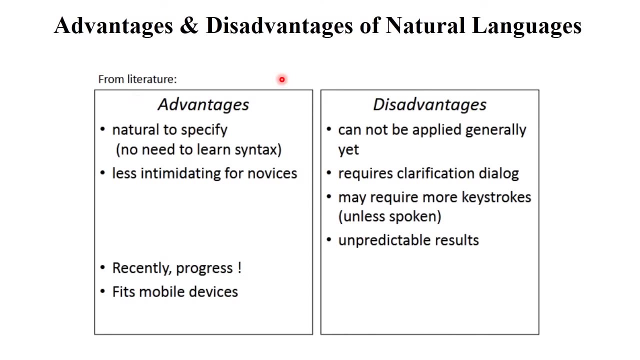 language. so source language is converted into the machine language. that's why we use different compiler interpreter for the conversion purpose. clear, these are the examples of natural language interface. next, again, there are some advantages and disadvantages of natural languages. advantages are natural to specify. no need to learn syntax here. 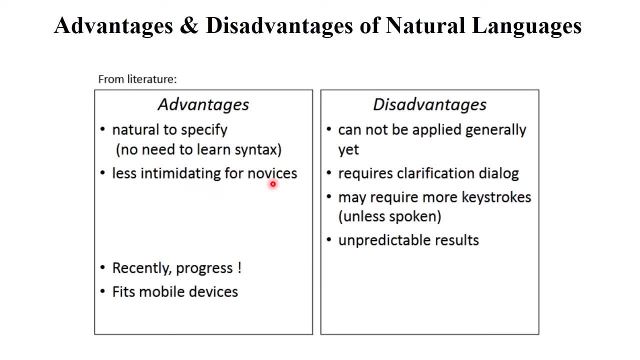 right then list intermediate for novices. it's easy to handle, for each and every person. recently progress and fits in mobile devices. recently there are various audio systems are available, clear, so it's easy to handle, but disadvantages are cannot be applied generally. it which is not apply for each and every system or each and every machineries. it requires clarification, dialogue. 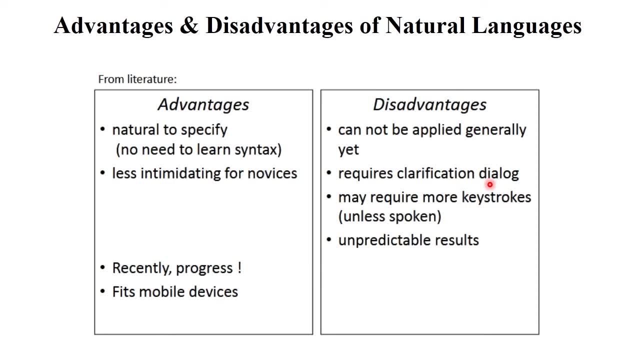 while using google audio, you have to use proper word for that purpose, or dictionary word. sometime. it may requires more keystrokes, unless spoken keystrokes means while typing you have to use keyboard. okay, so when you press the key, there are different keystrokes are generated. it requires more keystrokes because it's your own language, an unpredictable result. you didn't. 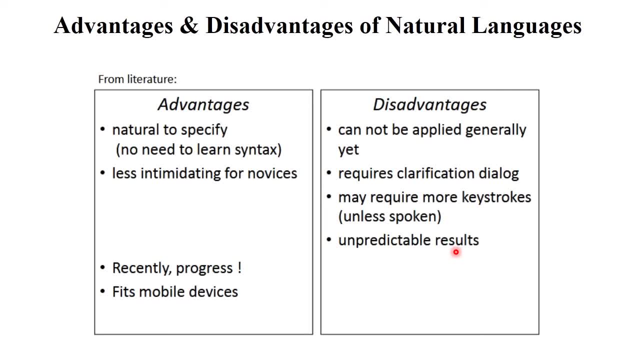 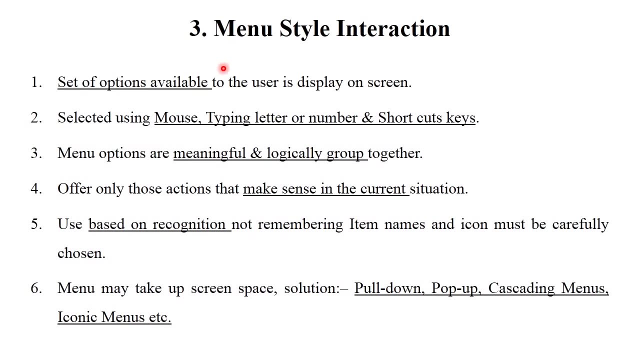 about your result by applying audio calls, voice calls, etc. clear. so these are the some disadvantages. this are disadvantages overcome in next interaction style- clear. next, the third interaction style is menu style interaction. we all are familiar with this menu. menu means set of options available to the user which display on screen it's selected. 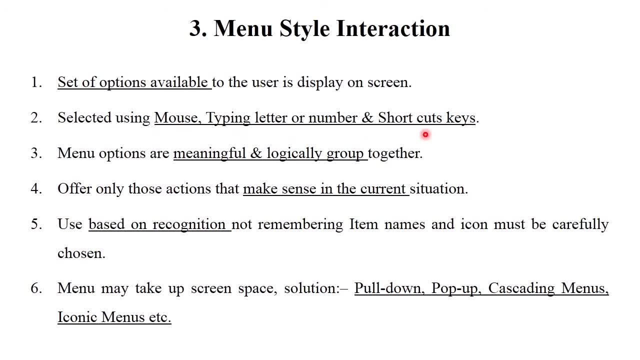 using mouse, typing letter numbers, and also shortcuts keys are available. menu options are meaningful and logically grouped together. it offer only those action that makes sense in current situation. it use based on recognition, not remembering. item menus are already given in menu bar. you didn't remember anything while using this, okay, or sometime each. 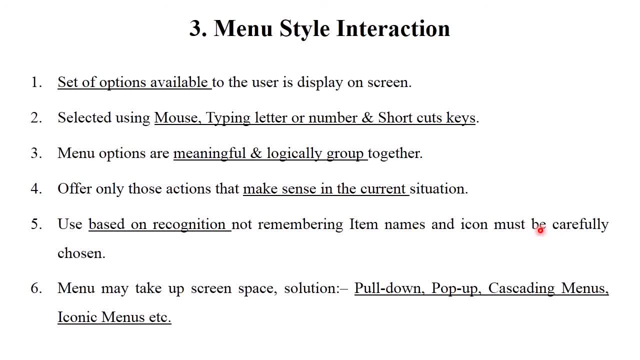 and every menu particular icons are given. you must carefully chosen each and every icon. the menus also have different types, like pull down menu, pop-up menu, cascading menus. cascading means, for example, there is a file option. in file there is new option, in new again there is. 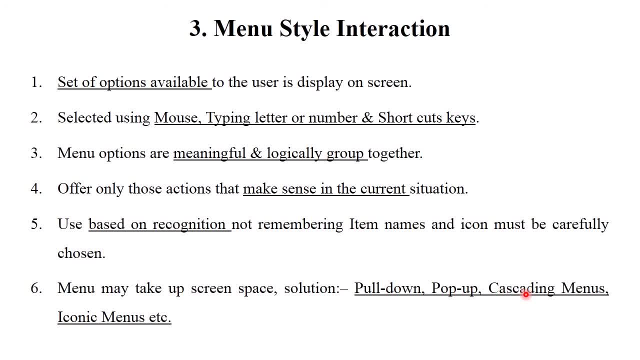 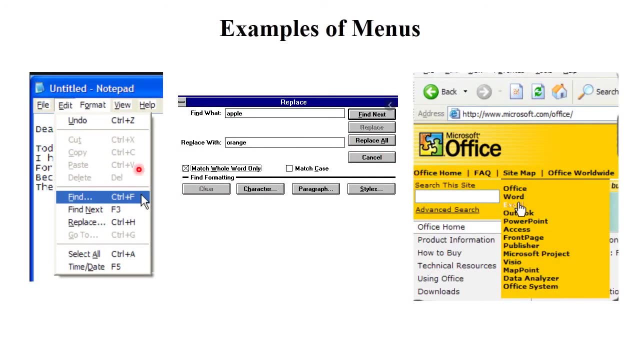 new option, right, so this is called as. cascading means interrelated- okay- and iconic menus. sometimes menus and icon is given clear. so let's take the example of menu style interaction next. these are the some examples of menus. we all are familiar with this. like there is notepad, Microsoft Word. 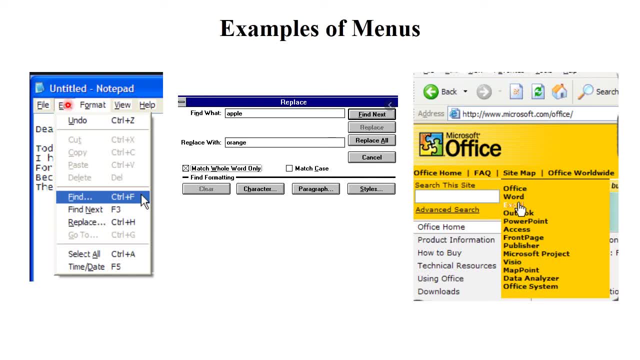 and PowerPoint or each and every application. the menus are given, for example here edit. in edit there are menus like cut copy paste, find next, etc. It means related, similar actions are combined or encapsulated with each other in edit. clear again, there are some advanced such, which includes office. 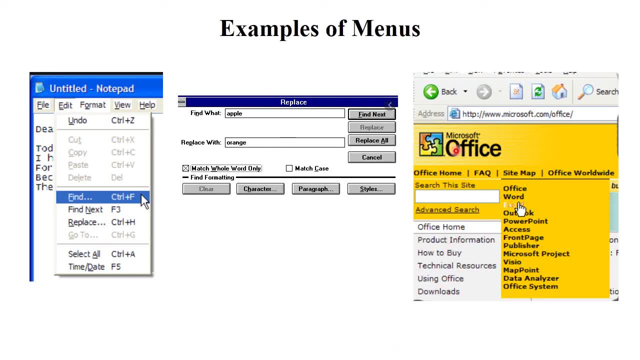 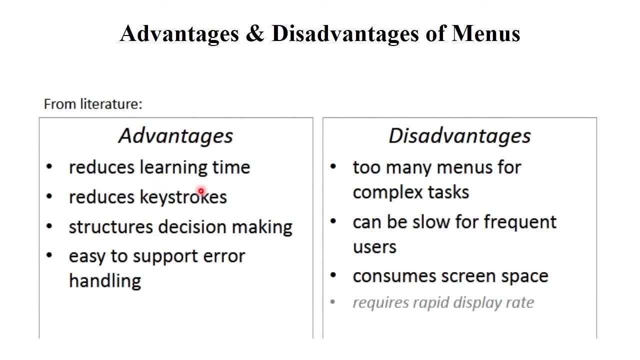 home, then office downloads, etc. so this is called as examples of menu, where menus are used which is easy to identify, logical grouping of menus, each other clear. next, the advantages of menus: interaction style. it reduce the learning time because it directly given. it reduce keystrokes, its structure. 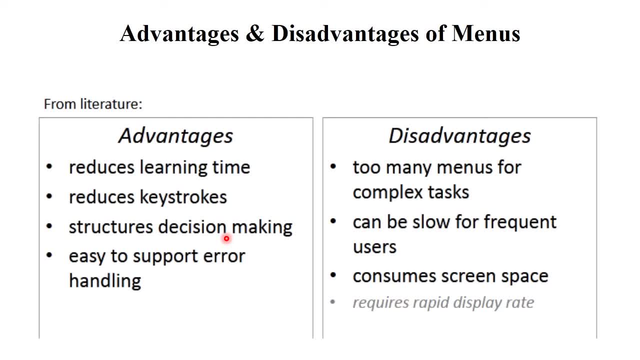 decision-making. proper structures or proper logical grouping or sequential groupings are there. it easy to supports error handling, okay. but also there are some disadvantages, like too many menus for complex tasks. if there are too many menu so it's very difficult to identify it, so you have to design the system on.